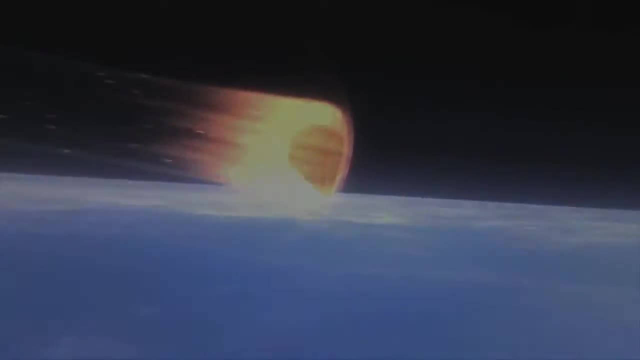 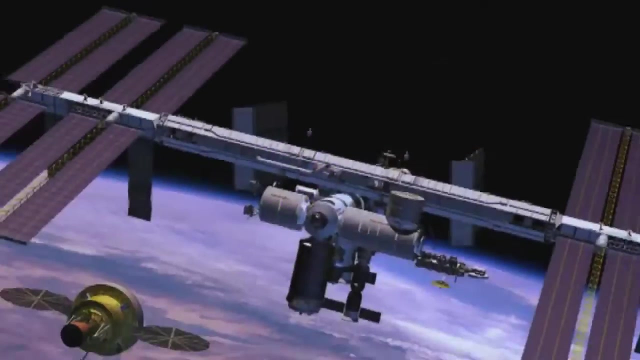 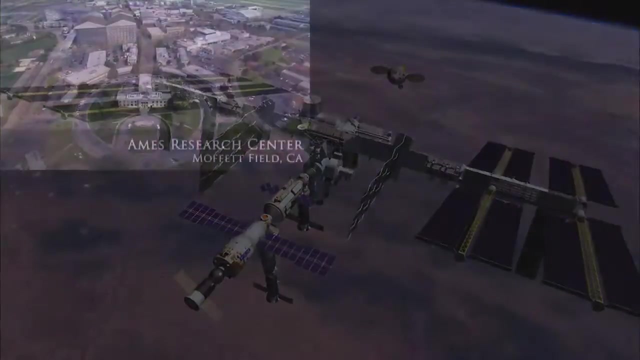 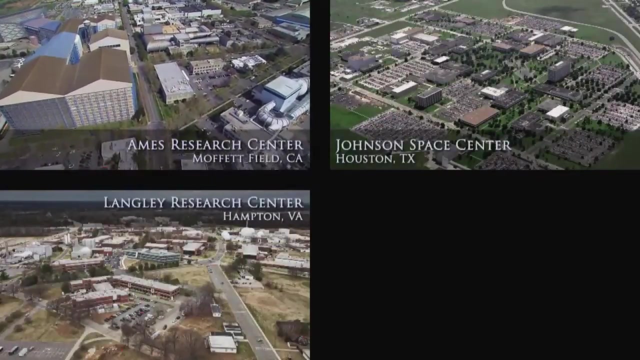 exceed the capabilities of current technologies. NASA is investing in the future with innovative and game-changing approaches to making thermal protection systems. Technologists from NASA Ames Research Center, supported by NASA Ames Research Center, are leading the effort in new ways of making thermal protection systems. 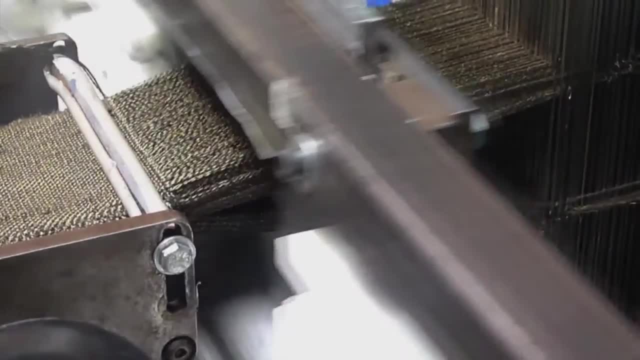 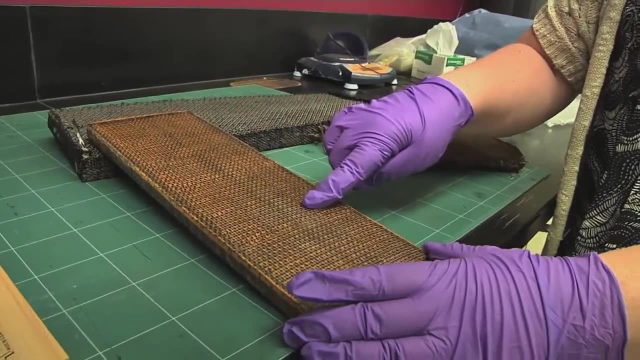 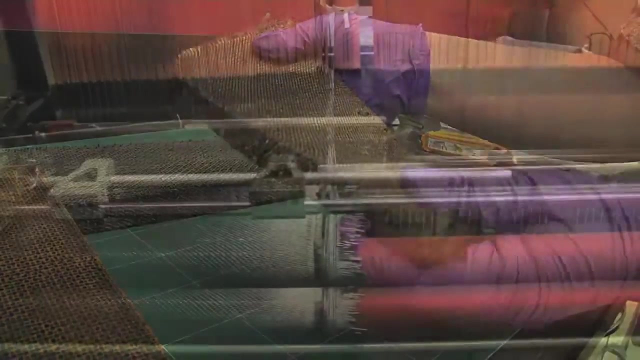 NASA is partnering with commercial textile producers and developing advanced automated weaving techniques to tailor and optimize performance. Weaving allows NASA engineers to manufacture both rigid and flexible materials that can withstand extreme heating conditions. Engineering creates an opportunity for best practices to be utilized that are sustainable. 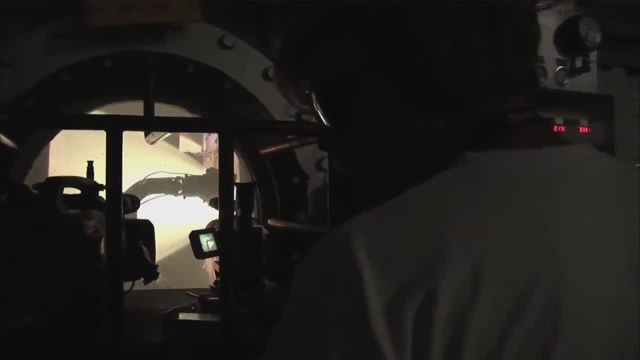 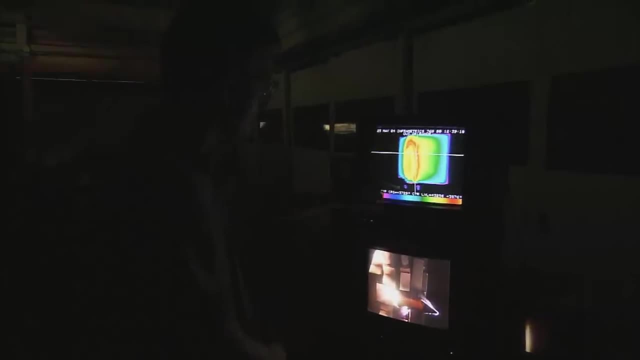 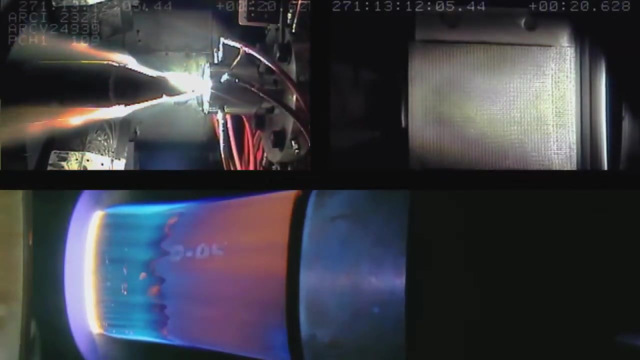 rapid and cost-effective To test new materials. special ArcJet facilities are utilized at NASA Ames and at the US Air Force Arnold Engineering Development Center in Tullahoma, Tennessee. Engineers use the ArcJet to simulate the high-speed flow of atmospheric entry and test the thermal. 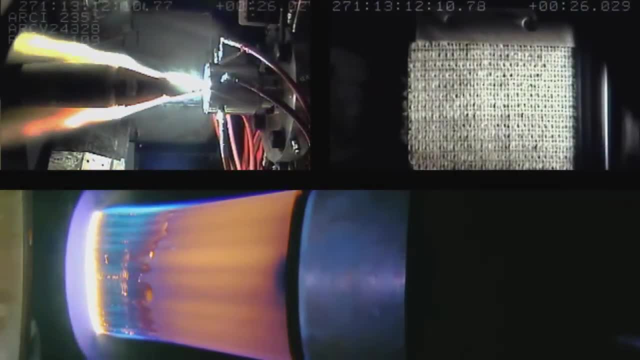 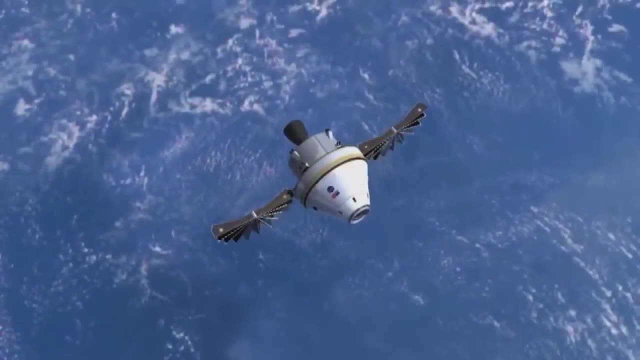 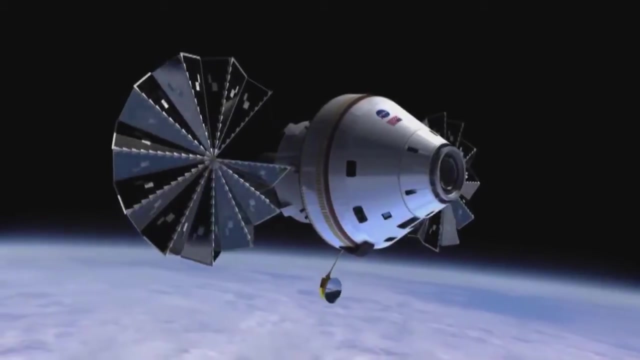 protection system at highly energetic conditions. 18 months ago It was just an idea: woven thermal protection system weaving a heat shield, and at this point we're already now in the stage of development where we're readying it for possible insertion into future human missions. 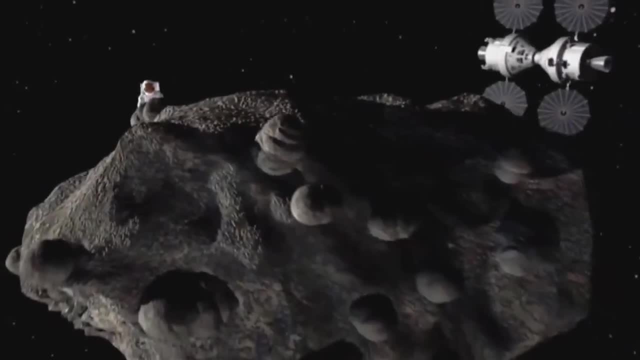 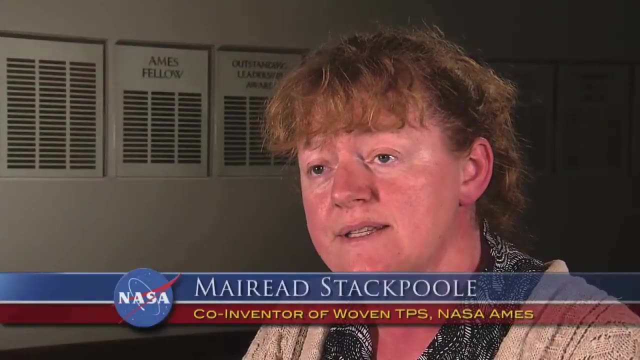 Using the woven technique, we're working to make a large heat shield that will allow safe return to Earth from a variety of NASA missions. Since weaving is an automated process, we can leverage that technique to design our TPS and have our TPS lightweight, robust and efficient. 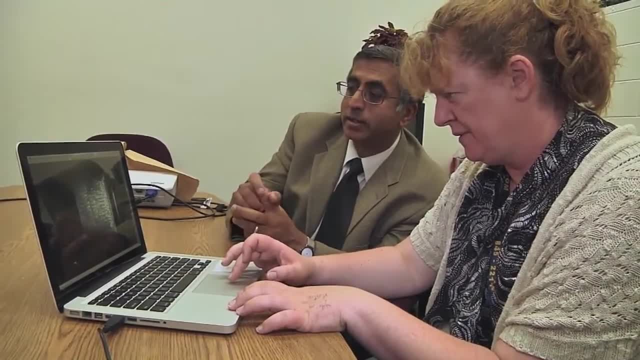 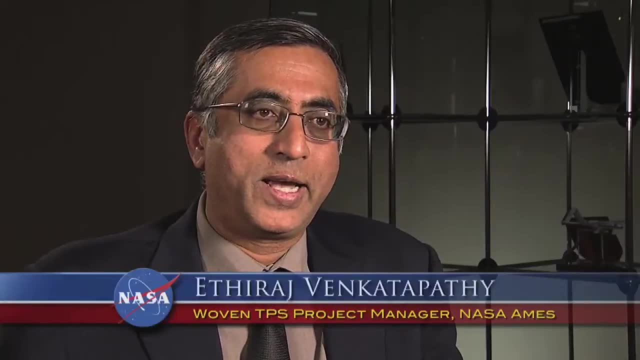 We're working to create a large heat shield that will allow safe return to Earth from a variety of NASA missions. It's a very rich and inexpensive technology. As an engineer, it's really great to work on technologies that are going to change the way of the future. 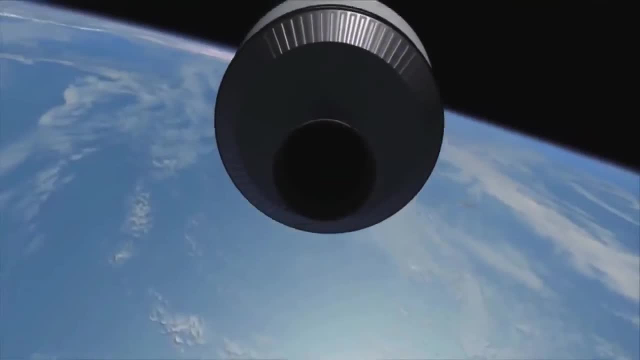 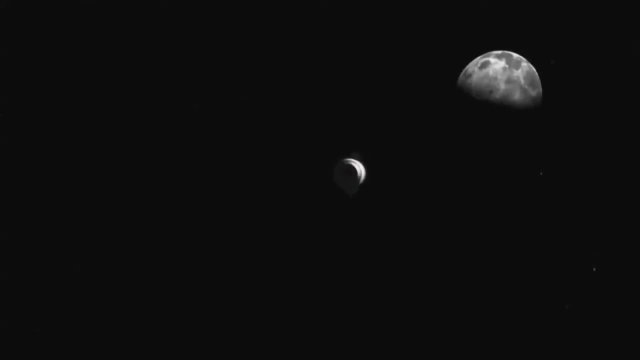 NASA today is investing in innovation and NASA Space Technologies Game Changing Development Program. it's helping to make future missions a reality. you.